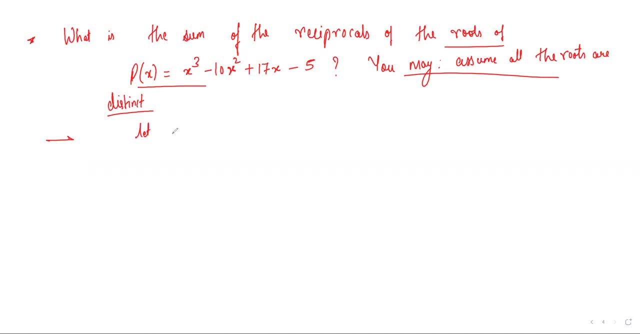 So let's try to solve this. So let A, B, C be roots of P of x. Now we need to find 1 over A plus 1 over B plus 1 over C, which is equal to A, B plus B, C plus C, A over A, B, C, right? 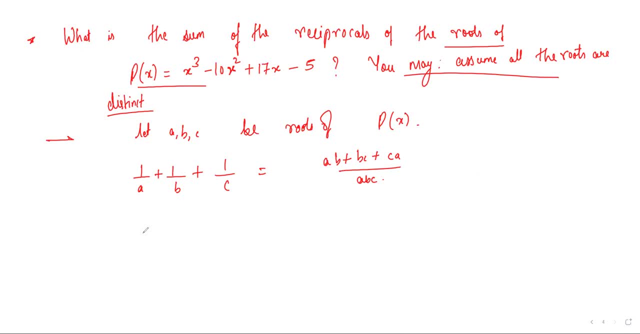 Now looking at the polynomial P of x is equal to product of the factor x-A times x-B times x-C, which is equal to x³, x³ plus x². So what's the coefficient of x²? x² will be minus A, minus B, minus C plus x times. 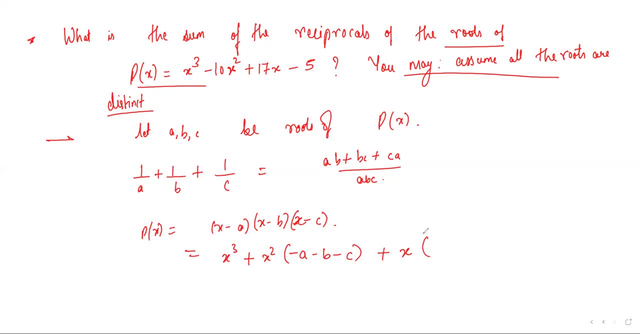 The coefficient of x will be A, B plus B C plus C, A plus A B C, So this is P of x. So from here we get that A, B plus B C plus C, A is coefficient of x. 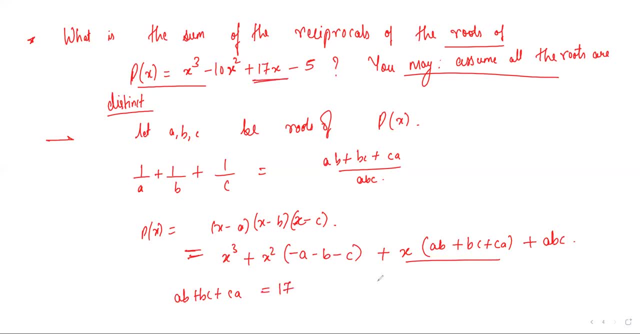 And the coefficient of x is 70. And A B C is equal to, So this should be minus. Sorry, So A B C. A B C will be equal to negative of the last term. 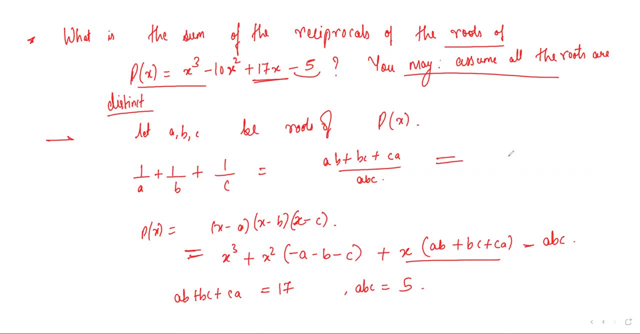 So A, B, C will be equal to. This term is equal to 70.. I hope the question is clear, Thank you. So, just to conclude, I end up the video with a question: Tell me what is A² plus B² plus? 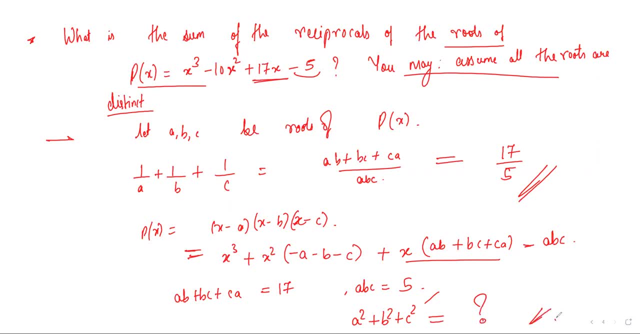